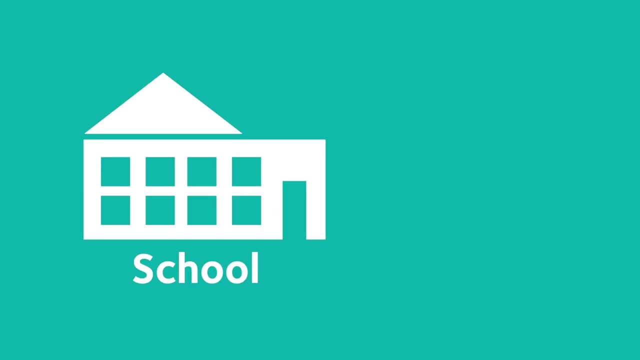 in mathematics that what happens is a lot of people can do their mathematics, that they do at school, but they haven't been able to transfer it over to the world beyond schools and so often when they're trying to make judgements about what's the best buy in the supermarket, 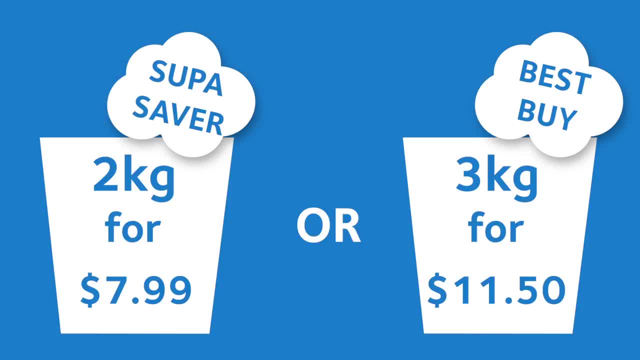 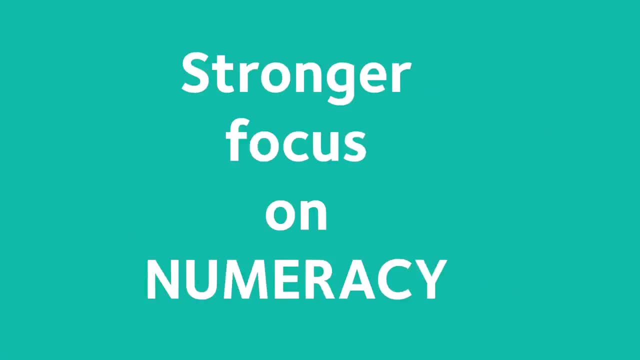 or should I take this home loan out, or all of those sorts of things that we face in everyday life. they don't use the mathematics that they need to use. So what has happened now is we're taking a much stronger focus on numeracy. But to be 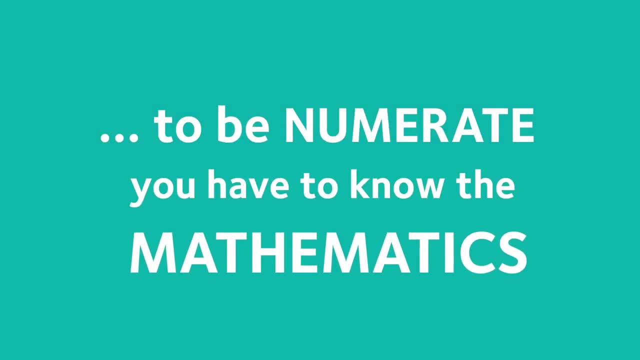 numerate, you also have to know the mathematics. So it's not much point being numerate if you can't add or if you don't know what mathematics to apply those sorts of things. So what we do now in mathematics is we have mathematics which is about the, what we call the esoteric. 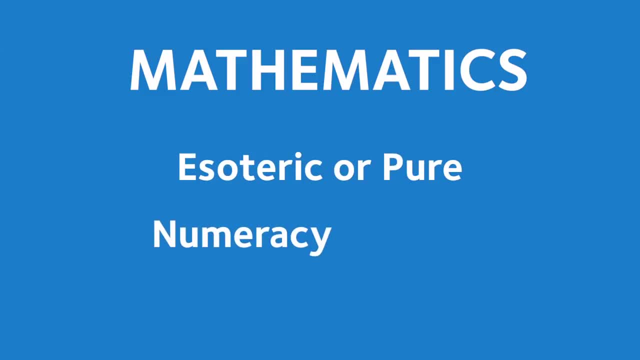 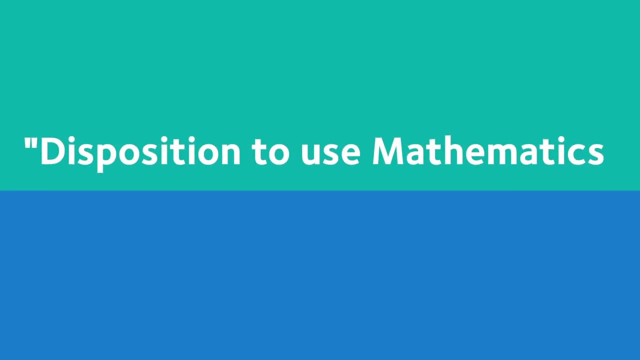 mathematics, the pure mathematics, if you like, and numeracy, which is much more the applied. The Australian association of math teachers actually taught a whole range of mathematics in the past. The Australian association of math teachers actually taught only one, or talk about having a disposition to use mathematics and mathematical ideas and mathematical processes. 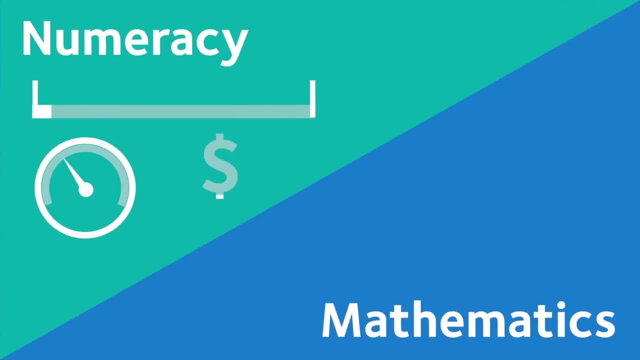 to solve everyday problems. So what you're going to find in this course and your subsequent course is- we're going to use these terms a lot. So in the informatics that you're just about to have a look at, what we can see are two different ideas. One is the numeracy idea and the other is the mathematics. 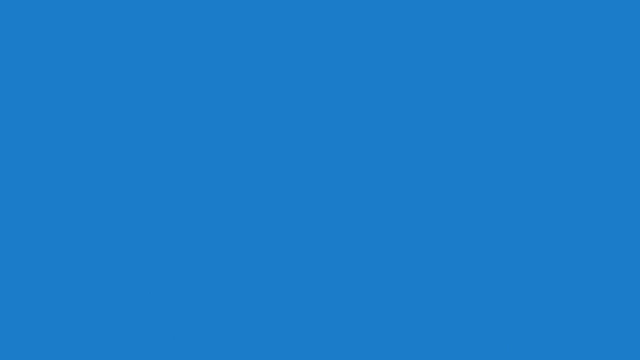 idea You might remember, when you were at school you did Pythagoras. you know, a squared plus b squared equals c squared, and that was how you'd find out the length of a side. because if you had a triangle that had a side that was three, three squares, which made a nine, and then the other side. 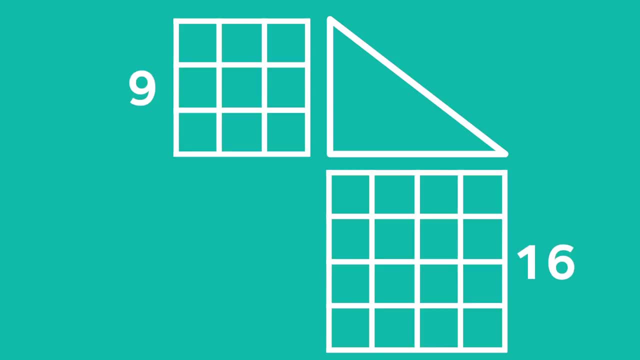 was four squares, which made 16. you have to find out the length of the hypotenuse, that long side that runs between those two angles. Now this only works, remember, for a right angle triangle. it doesn't work for all other triangles. So while you're at school you probably had to play with 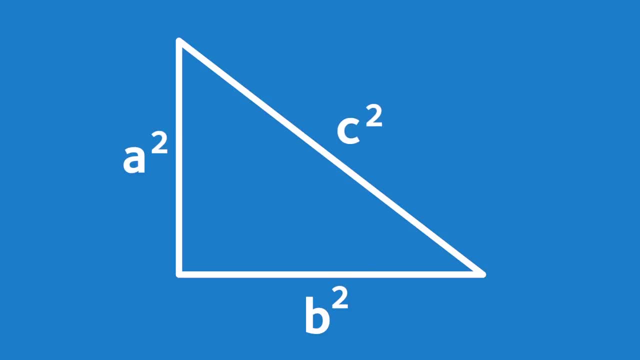 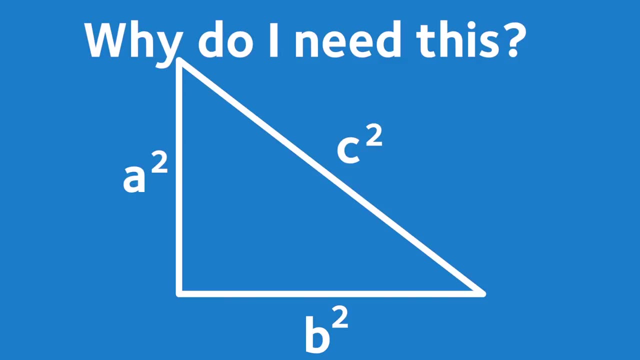 a squared plus b squared equals c squared, and you never learned aboutloration, never realized why you would need that, other than to solve problems in school and out of your textbook. however, what we do know, and so that's that's mathematics. but what we do know is that 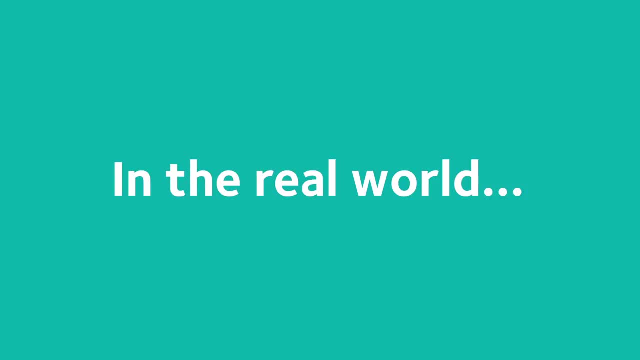 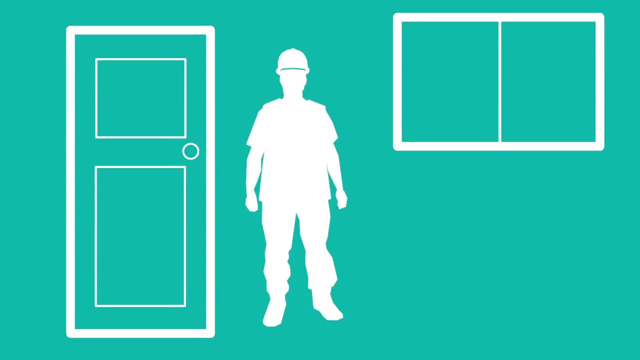 if you work in the real world, in the world beyond. school builders need to know that if they're building something, and they're building, say, a door frame or a window frame, they need to know that square so they might have a square, an instrument, but they also know that they have 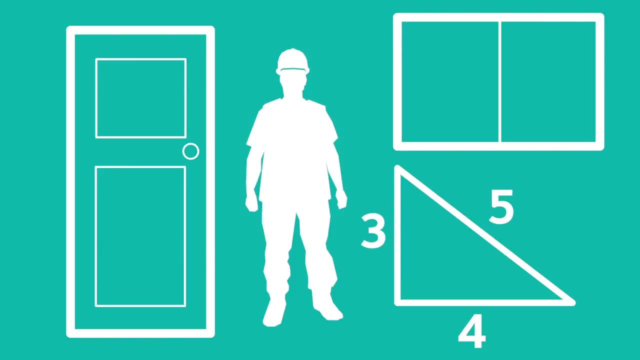 this thing called a three, four, five, and if they've got a three, four, five triangle, so one side's three let units long, whatever that might be, the other is four units long, and so long as the hypotenuse is five units long, that corner where the three and the four meet is actually going to be very 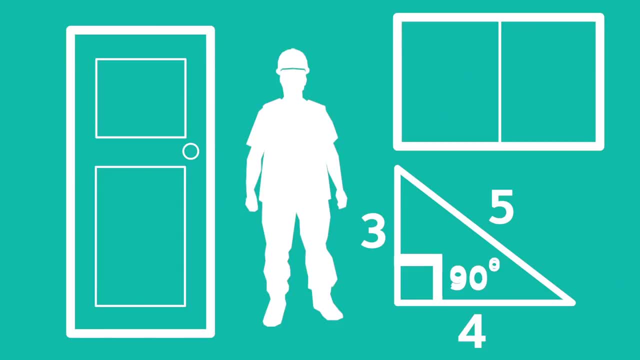 square, so many builders use that notion. so, in actual fact, what they're doing is they're using pythagoras that they learned at school in everyday context, and using it very, very successfully. they won't call it pythagoras, they'll just call it a three, four, five. so this is the difference. 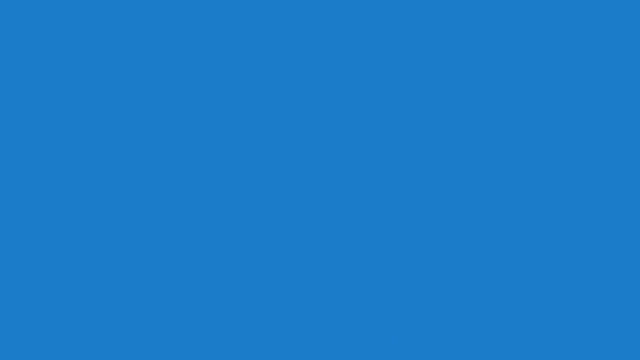 between numeracy and mathematics. now, another thing that we know is that when we teach subtraction, for example, one of the biggest problems we have in maths is when we have to subtract numbers and there's zeros, internal zeros. so if you give a problem like 5.00, subtract or take away or minus. 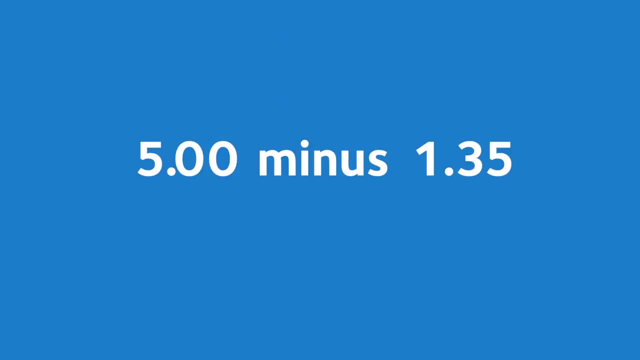 whichever word you would like to use: 1.35. a lot of people will say, oh, i don't know how to do this and they might start to panic. so we start to put it down in in laying it out in the column. so we have on our first line, we have: 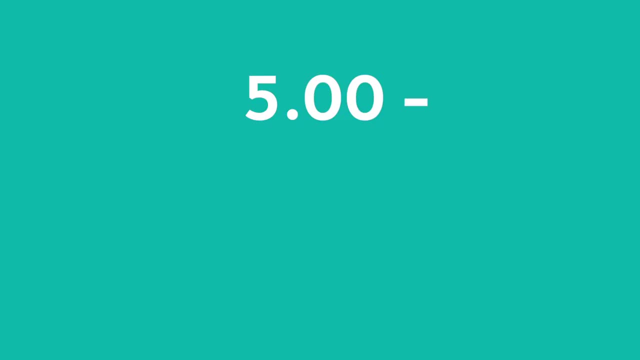 five point zero, zero. then we put our subtraction sign and then, directly underneath all of those numbers, we go through a process where the one is directly below the five and the decimal points line up, and then the three and then the five. then we have to start taking them all away. 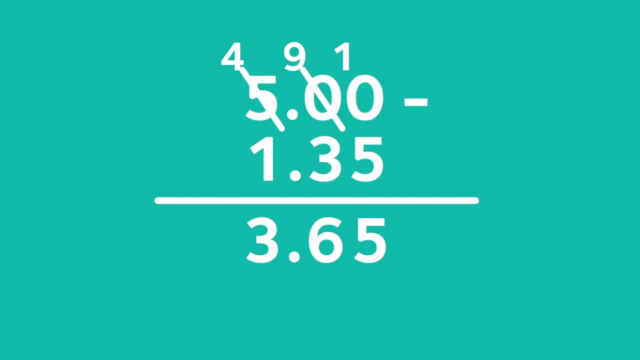 and you probably remember that process. now we know that kids get this wrong. that will take it all away incorrectly and they have no real understanding of what they've got to do. hopefully, if they do a check afterwards and they add the bottom the the answer up with the 1.35, it'll add up to 5.00.